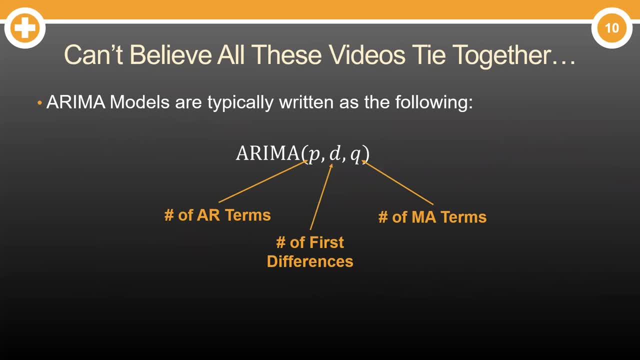 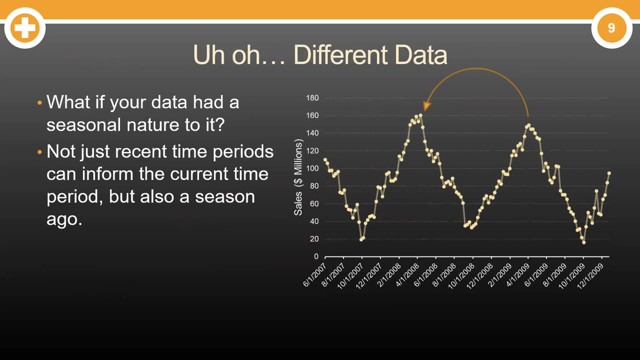 written, as you see here, with three numbers that summarize them: P- the number of AR terms, D- the number of first differences and Q- the number of MA terms. But what if? What if your data actually had a notion of seasonality to it? Energy fluctuates depending. 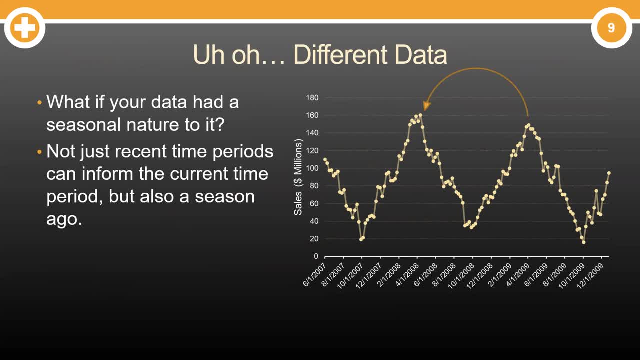 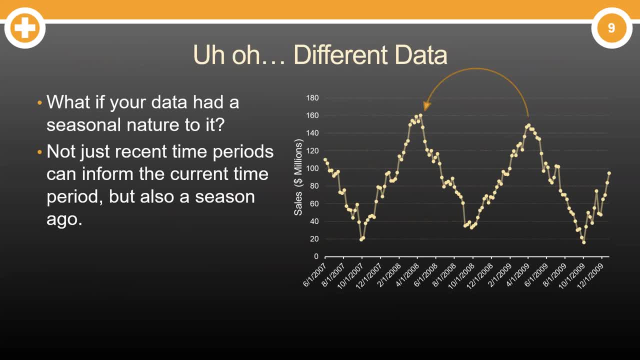 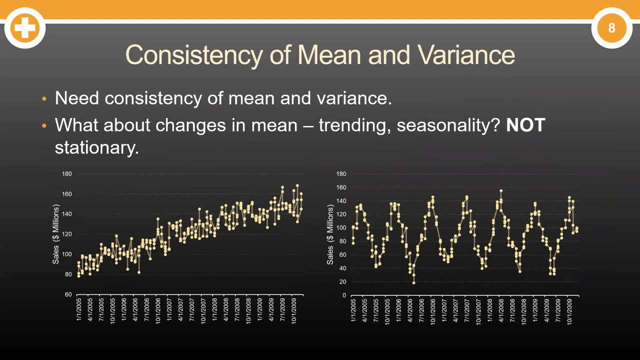 Or an MA error lag effect. But be careful, Remember that ARIMA models are stationary models. Yep, going back down memory lane, Remember seasonal data is not stationary by design. Again, click on the link in the upper right-hand corner for a refresher on stationarity, Sorry. 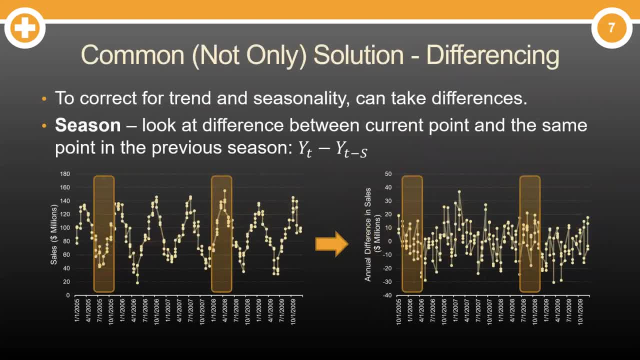 these videos are all connected. However, we can take differences. It isn't the only solution, But it is a common one. This differencing will make our data stationary. However, that doesn't mean you have removed the seasonal correlations. What happened? One season's number? 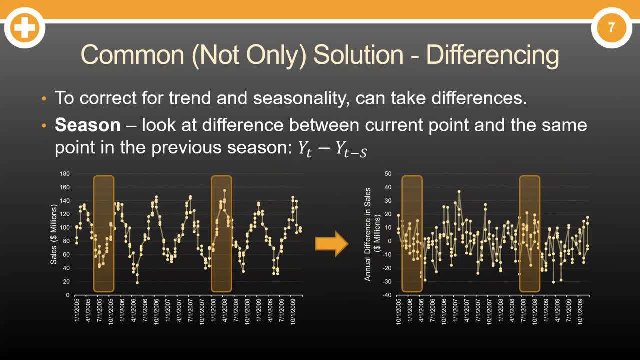 of data points can still impact the current data point, And that's great. So our data looks a lot more stationary, but we still have the underlying patterns that still exist. Excellent, This leads to the creation of the seasonal data point, And that's what we're going to do. We're going to 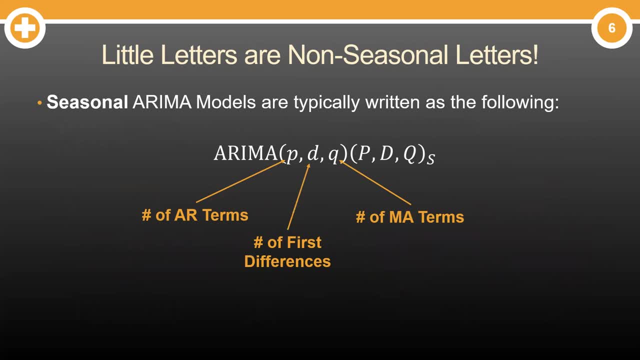 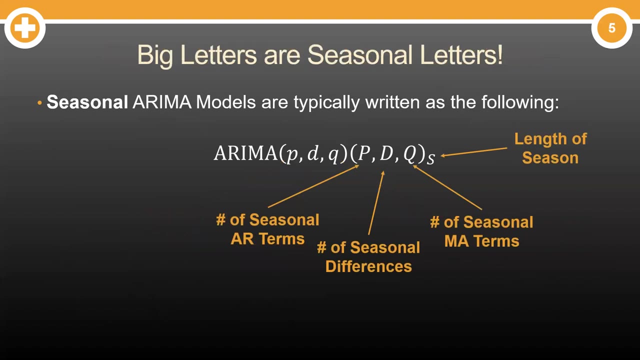 create a seasonal ARIMA model. We still have the regular ARIMA pieces. Little p represents the number of AR terms, Little d the number of first differences. Little q, the number of MA terms. However, we now have the seasonal components to the model as well. Big P represents the number of 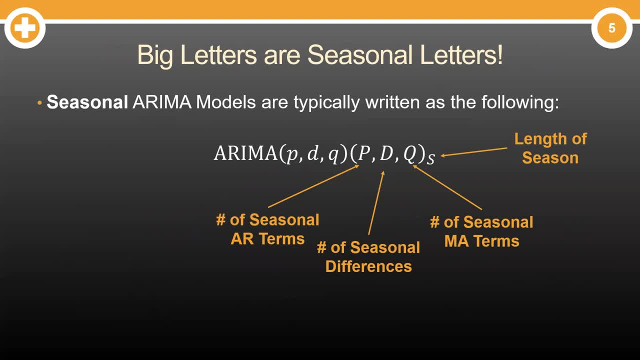 seasonal AR terms. Big D is the number of seasonal differences. Big Q is the number of long term seasonal differences. Big K is the number of current achieving. So we don't have this part of the deal of seasonal moving average terms. How big is this season? 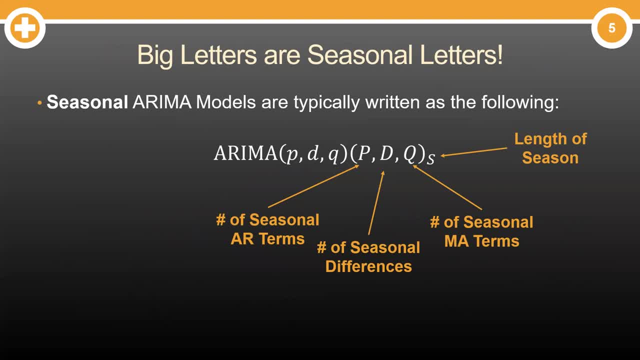 In other words, how many data points are in each season. That is what S tells us. All right, let's finish this up with an example. Can you write out what this model would be in a REMO 101 to 1012??